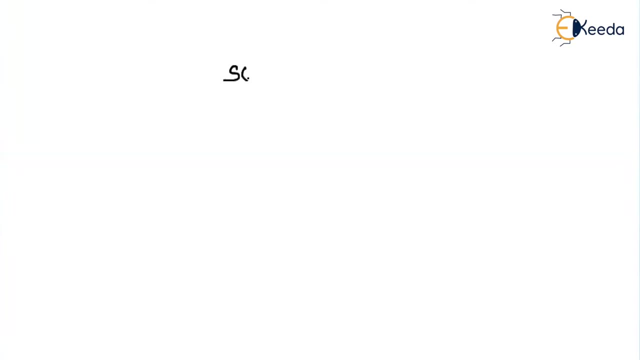 Now let us consider, suppose, if I am having some soil, so in first, in how many categories I can divide this into. okay, so I can divide this into three different categories, and first one is coarse-grained soils, coarse-grained soil, and second one is called fine-grained soil, fine-grained soil. 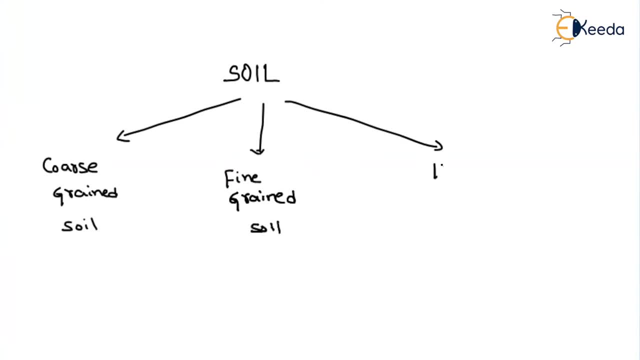 And third one is highly organic soil. highly organic soil, highly organic soil. okay, So the name itself, coarse-grained. that means we can, by listening that term, we can say that the size of the particles are little bit in larger in comparison to the fine-grained soils. okay, 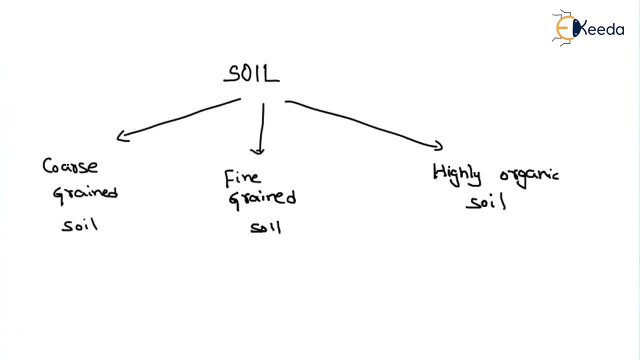 And organic is it is like due to because of the some wastages. okay, So let us see: how can we classify? How can we classify a soil into coarse-grained, into fine-grained soil? Suppose, if I am taking a soil, let us say if I am taking a soil and I am considering, let us say if I am taking some amount of W and I am passing this soil through the sieves. 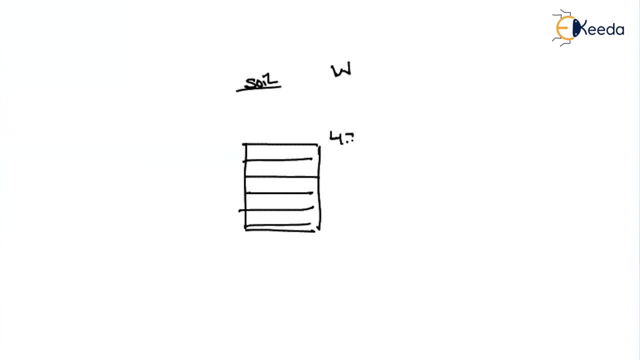 So what are the maximum and minimum sizes? So here we will: at the top we will have this 4.75 mm and at last we are having the 75 micron, And below we are having some palm right. 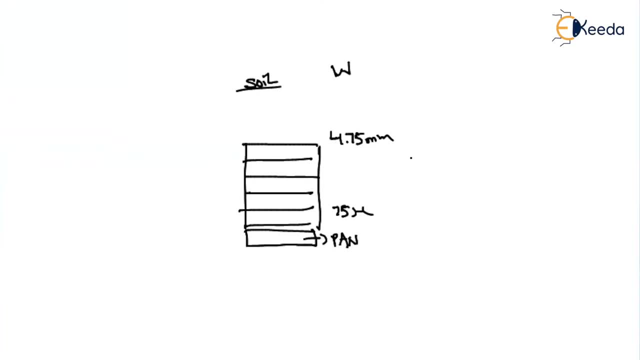 So if your soil is retained, whatever the soil is retained in between 4.75 to 75 micron, we will classify that as a coarse-grained soil. Whatever the soil that is retained, or the size less than the 75 micron, we will call them as a fine-grained soil. 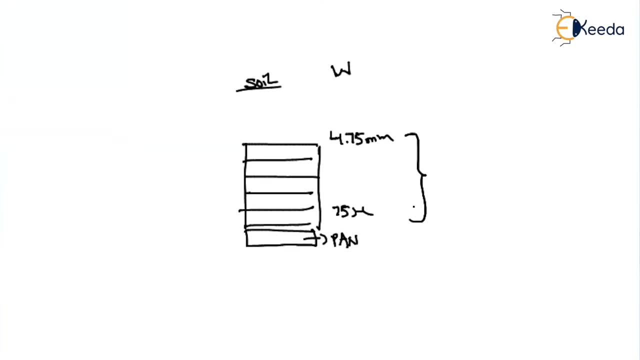 But overall, how can we say if I am taking some soil, how can I say Is it a coarse-grained or how can I say it is a fine-grained soil? It is obvious that if the percentage of the soil is more in between 4.75 to 75 micron, then we will classify that as a coarse-grained soil. 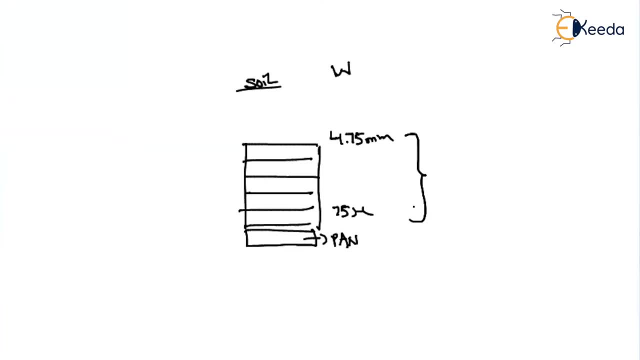 And similarly the soil retained on the palm. if it is greater than the 50%, then we will classify it as a fine-grained soil. That means further. let us take, Let us take an example. So here I will tell you only two different sieves. 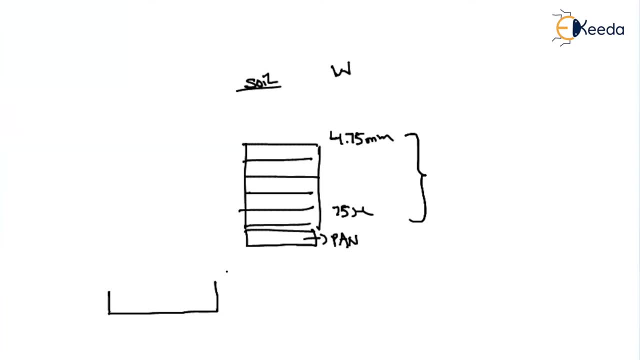 That means I will say this is a 75 micron. So let us take that only 4.75 micron sieve and pass the soil through 75 micron. So whatever the soil is retained, Whatever the soil is retained If it is greater than 50%, 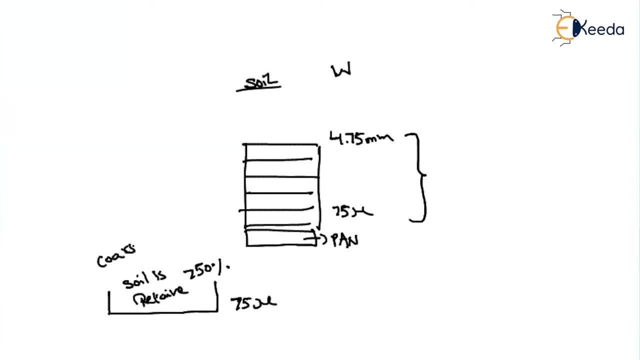 Then we will classify it as a coarse-grained soil. So whatever the soil that passes through 75 micron. if this percentage is greater than 50, then we will classify it as a fine-grained soil. So the percentage- if it is greater than 50%- passes through the 75 micron, then we will classify it as a fine-grained. 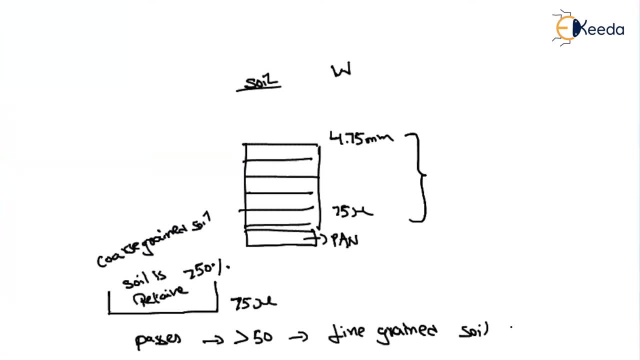 Whatever the soil is retained, Whatever the soil is retained, Whatever the soil is retained, Then we will classify it as a coarse-grain soil. So let us say this is a Soil. Let us say: if I am passing through the sieve, 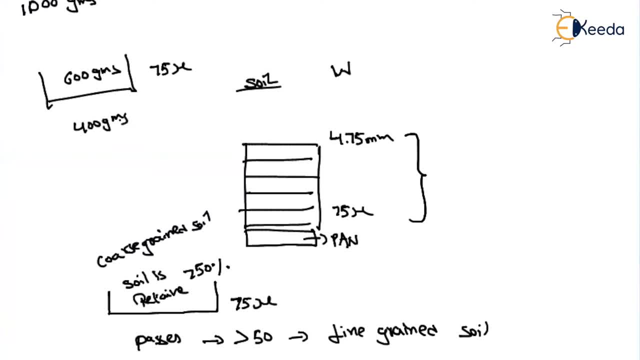 Let us say that 600 grams, Let us say that 600 grams, Let us say that 600 grams, the 75 micron. so what is the percentage of the soil that is written on the 75 micron out of the thousand? how much is retained? 600, so how much? 60 percent, so how much portion is? 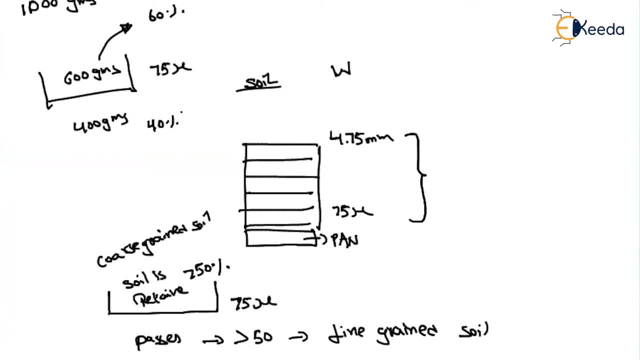 passed through the 75 micron, that is nothing but a 40 percent. so which percentage is more? soil which is retained on the 75 micron is 60 percent. that's why it is classified as a coarse grained soil, so the soil is retained, passes the 75 micron is 40 percent. so it as it is less than. 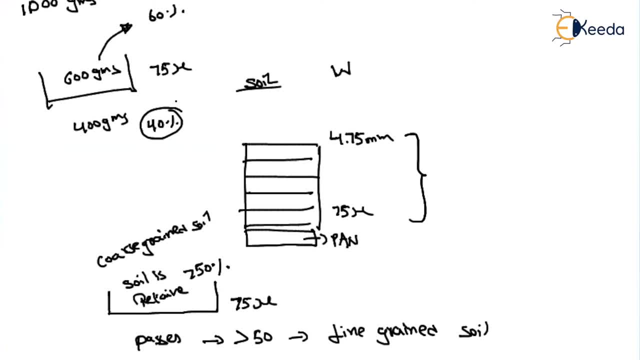 50 percent, then we can see. so if it is retained on the 75 micron more than the 50 percent, then we will classify it as a coarse grained soil. if the soil passes more than 50 percent through 75 micron, then we will classify it as a fine grained soil. 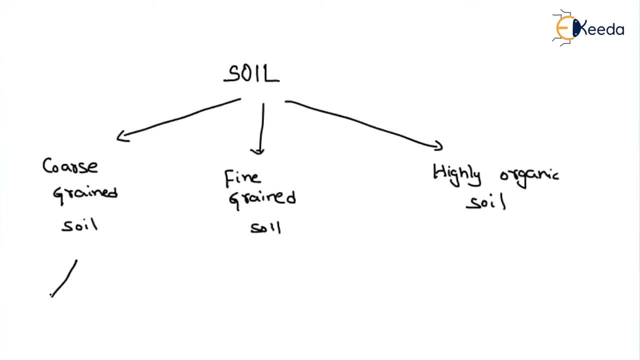 and again, if i see further classification, then in general. first, my coarse grained soil is divided into gravel and also divided into sand. similarly, if it is a fine grain soil, we have divided this into silt and also we have divided this into gravel- sorry, silt and clay, and also 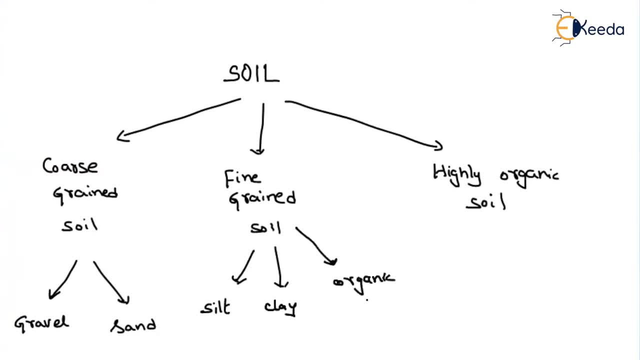 we are defining it as a organic soil. see, if it is organic soil, then we'll say it is a fine grain, but if it is highly organic, then we are saying it is a separate classification. so, gravel, this is represented by the term capital g. sand is represented by the symbol s. silt is represented. 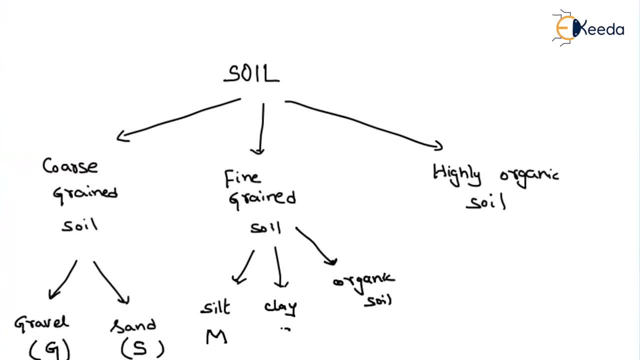 by the symbol m. clay is represented by the symbol c. organic soil is represented by the symbol o. highly organic soil is represented by the p, subscript t. so generally these organic soils are possessed very dark color. so there is organic soil, so we don't use it for any construction purpose. 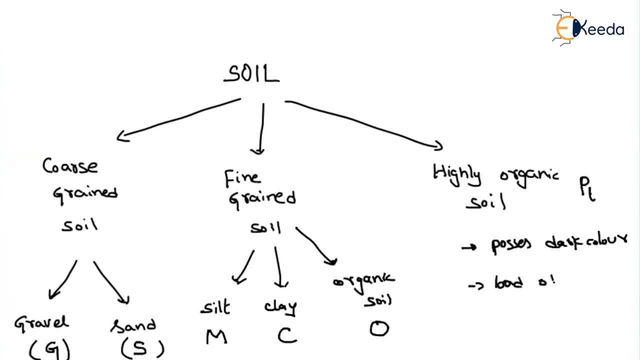 so as it is highly organic, that may produce some bad order also. so by depending upon these two, we can simply say whether it is organic soil, or whether it is highly organic or not. so example, please: we can say it is a peat, so as the soil formation under as they are removed from the 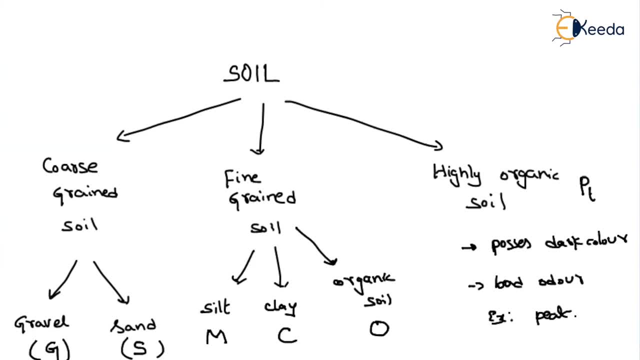 gate syllabus, so we are just defining this term. if that portion is there, then we could have discussed about the what are the types of the soil, how they are formed under, but for the 2021, that is not required. only you should know that. how to classify a soil system, that is more than enough. so this is. 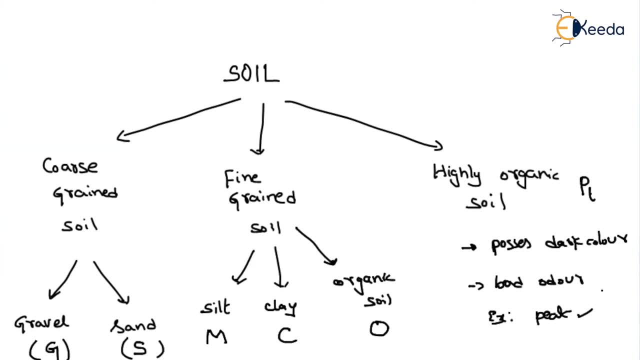 how we will briefly classify the system. that means we can divide into coarse grain, fine grain and highly organic. under coarse grain as further, we are dividing it to gravel sand, and if it is a fine grain, again we are dividing it to silt clay, organic soil. okay, now let us see. 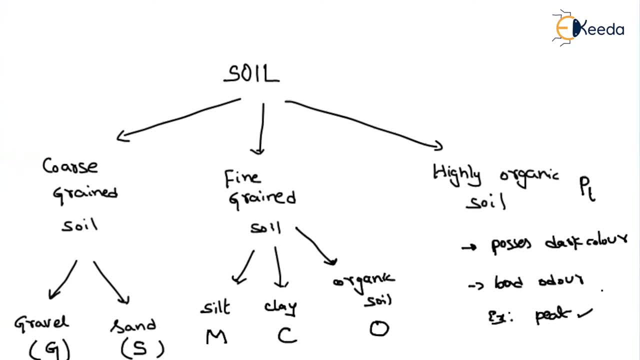 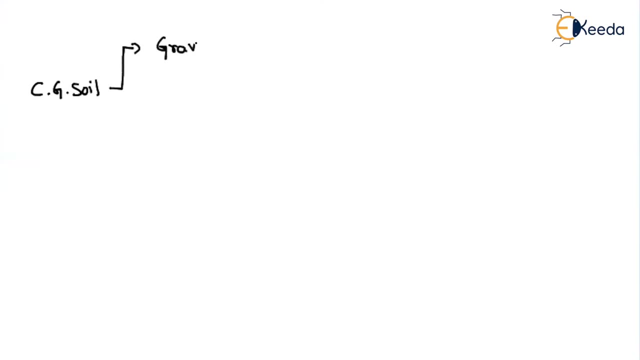 how we will classify again the gravel into and again how the sand will classify. as we discussed, coarse grained soil is divided into. we have divided this into gravel and also we have divided this into sand. so whatever the symbol for gravel g, whatever the symbol for sand s, so again this gravel. 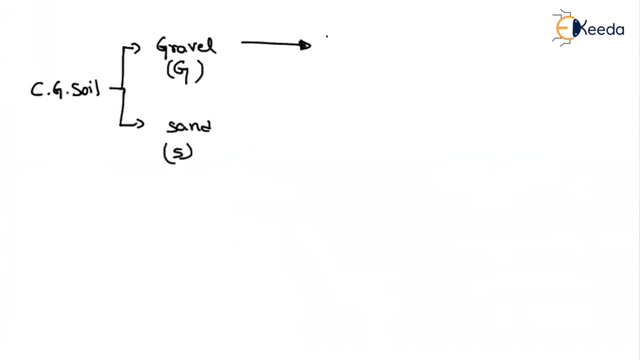 is divided into four different ways. that means first one: it is nothing but a well graded gravel. already we have defined what is meant by well graded in the previous lectures and and we have also divided this into poorly graded gravel, poorly graded gravel. and also we have divided into silty graded gravel, silty graded gravel. 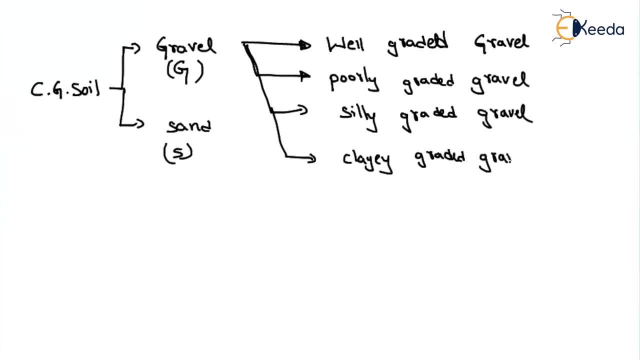 and also we have divided still this into clayy graded gravel. So well graded gravel we are representing by the symbol ZW. So make it like a mirror image. wherever you identify the symbols, imagine a mirror image. Well, what is the mirror image? point W: that means. so those are mirror image, well graded. 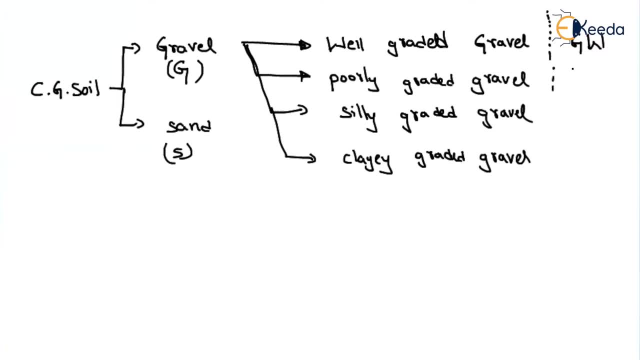 gravel Always studied from the right side to the left side. Okay, So poorly graded gravel gravel represents the G. poorly represents the symbol P. That means poorly, just study, like this poorly graded gravel. Similarly, depending upon these two, how can you define this silty graded gravel? so what? 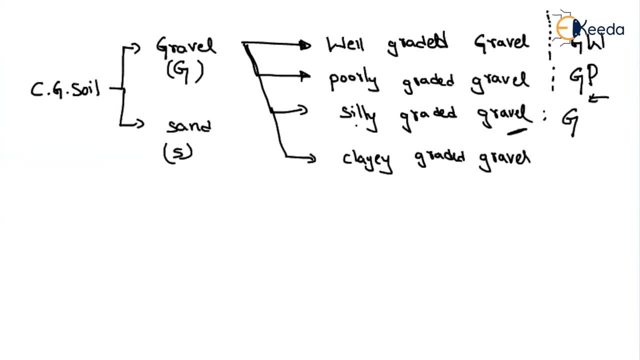 is the major portion gravel. So for the gravel G, silty graded. what is the symbol for silt? M? So silty graded gravel. Similarly, clayey graded gravel, that means G, C, Okay, Okay. 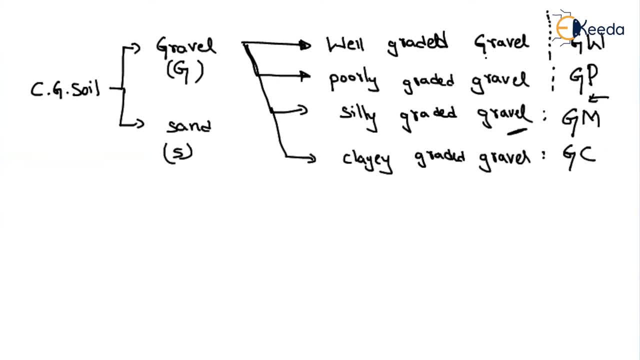 So always remember that. see, it is a well graded gravel. let us see this clayey graded gravel or silty graded gravel. Let us see if I am talking about silty graded gravel, That means, by listening this term, we can say that my silt content, my silt content. 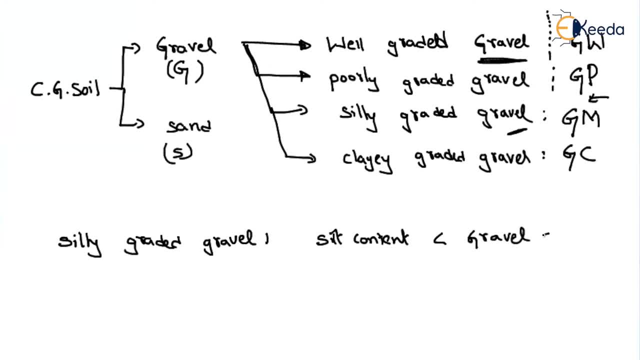 in the soil is less than the gravel content. So the main classification is this: Major classification is gravel, but depending upon the fine grain portion. so as a silt content is more, then we can say that silty graded gravel. That means major classification is gravel, but in sub still we are saying it is a silty. 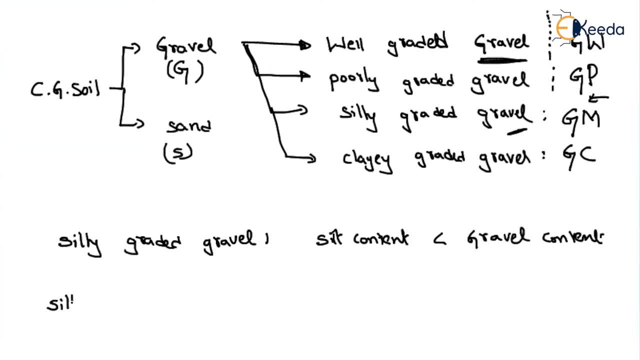 graded gravel, Suppose. if I am saying it is a silty clayey gravel, then what you can say, which portion is larger? So always the end term represents the major soil. Okay, Okay, Okay, Okay. So what we can say? we can say that silt content is less than the clay content is less. 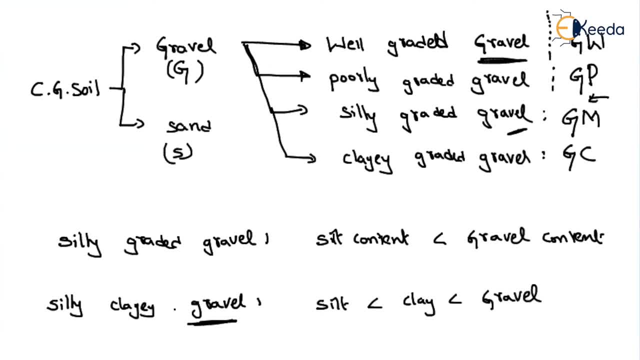 than the gravel content. So it is nothing but a coarse grained soils, understand. So this is how we will classify the gravel. Similarly, can you tell me how can I classify the sand? Again, we can classify it into four different ways. 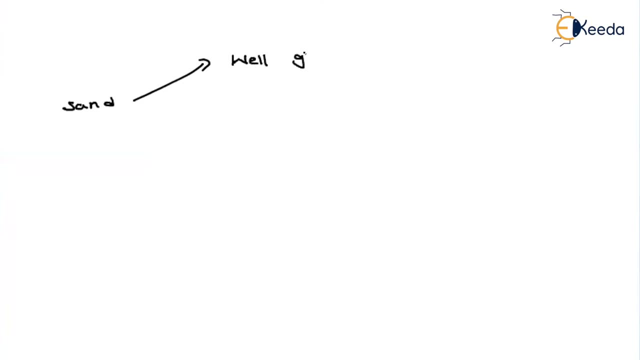 What are they? Well graded sand. Well graded sand, So what is the major soil Sand? Well graded sand, So what is the major soil? Sand? So sand means s well graded, So well represents subscript. 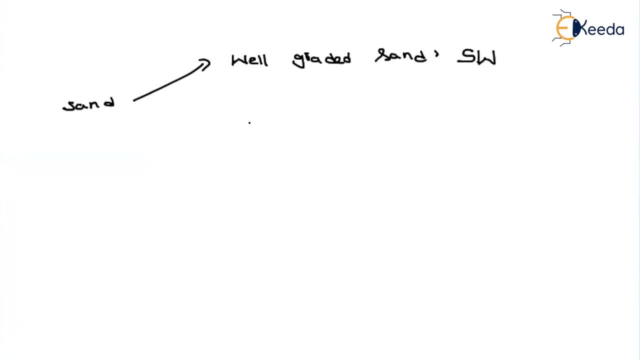 Similarly poorly graded sand. Poorly, what is the term P here? So poorly graded sand. Similarly silty sand. So which is a more major content? Silty or sand, Silty, sorry sand. So that is what it is. 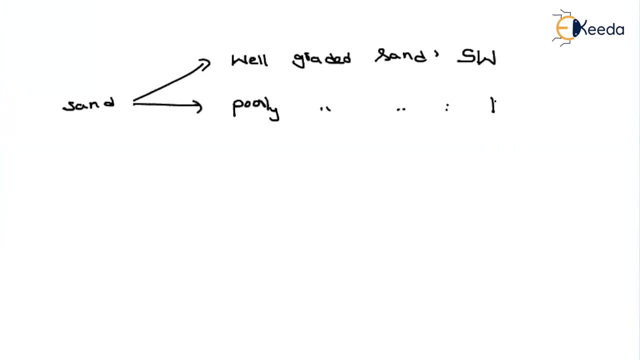 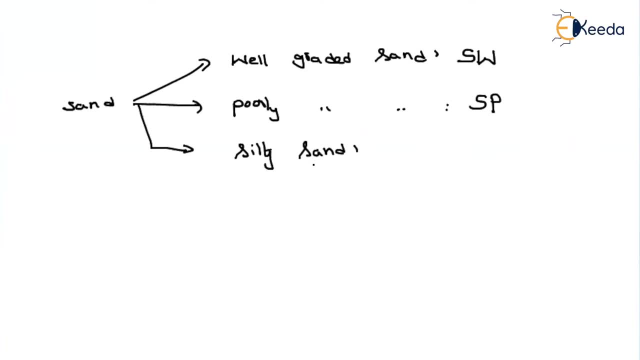 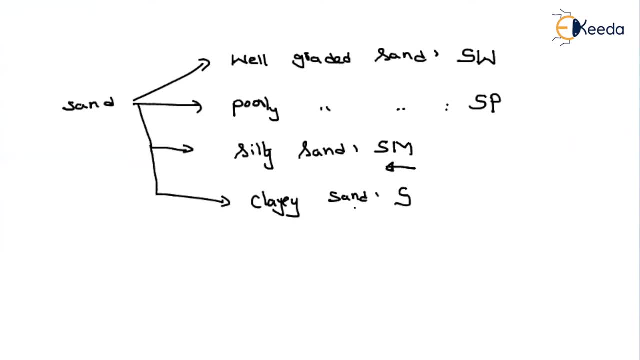 Silt, Silt, Silt, Silt. kal πrCHO RCO kQ'2. cYes Is, it makes me li. H2- Opposite, h2 Propuced kW. Oomp, So around 2 n. 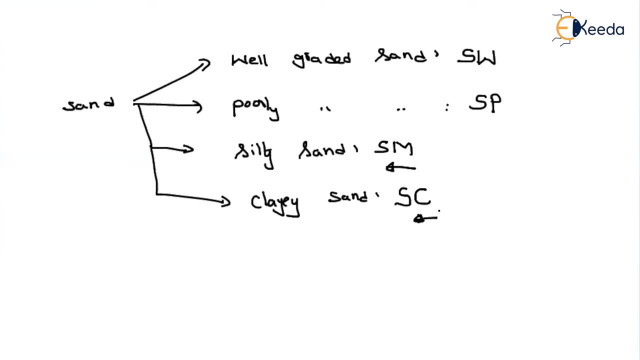 h, h3, g, hu, hx, h2, t, o, e, o sand. also, we are depending into four ways. so let us see: how can you say whether it is a well graded gravel and how can you say whether it is a poorly graded gravel under? okay, so as of now, what we know, 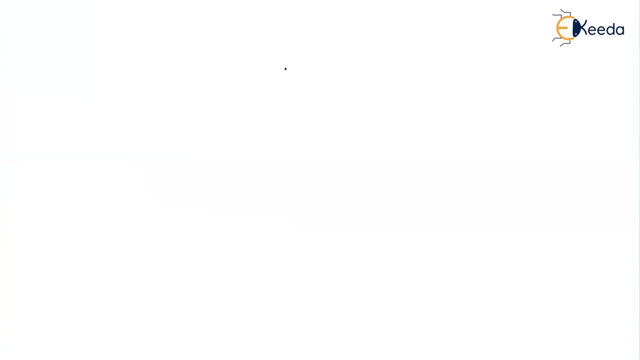 we know that if we are taking a w grams, if we are taking w grams of the soil, then if, out of this w grams, if soil retained, if soil retained on 75 micron sieve is, if it is greater than 50, then we are classifying it as a coarse grained soil. similarly, if soil passes through, 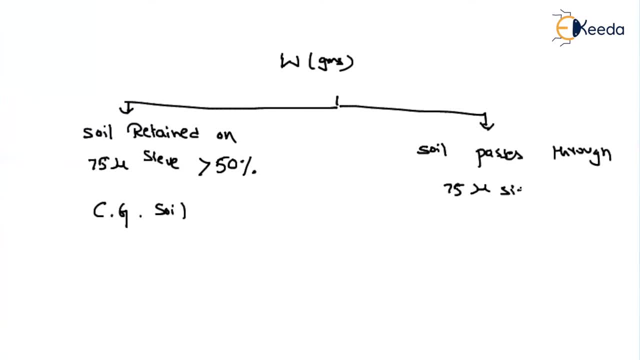 75 micron sieve is greater than 50 percent, then we are classifying it as a fine grained soil. now again, let us see again. the coarse grain soil is further divided into gravel and also further divided into sand. so let us see out of those first. let us see first. we have 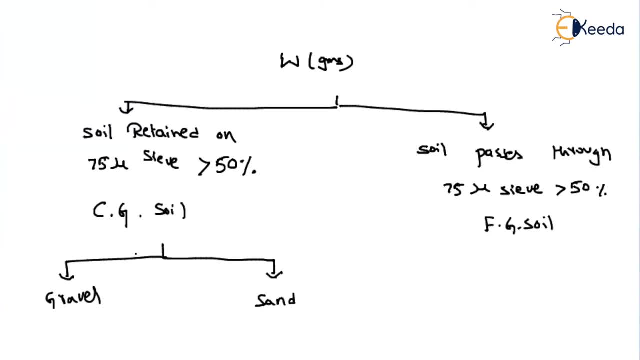 to identify whether it is a gravel gravel soil or whether it is a sandy soil. so for that, now let us consider the sieve analysis. now we have observed that it is a coarse grain soil. we have already discussed what is meant by coarse grain soil. so if i see all the sizes, 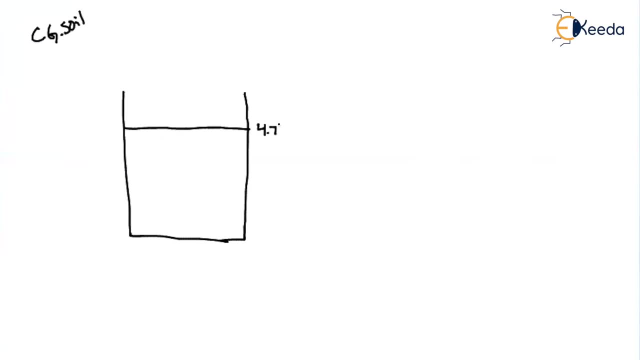 so what is the limit for the gravel? it is nothing but a 4.75 mm, 80 mm to 4.75 mm. then how will you classify the sand if it is 4.75 to 75 micron, isn't it? so, whatever the soil that is retained on the 4.75 mm, if it is greater than 50, 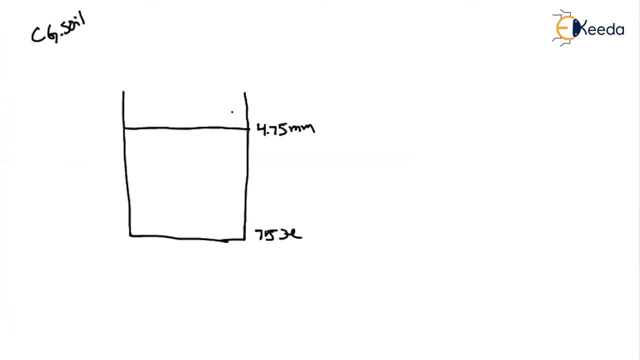 then again we will classify it as a gravel. so the soil soil retained on 4.75 mm. if it is greater than 50 percent, then we will classify it as a gravel. and how will you classify a sand then? how will classify it? we will classify it. soil passes through 4.75 mm. soil passes through 4.75 mm. 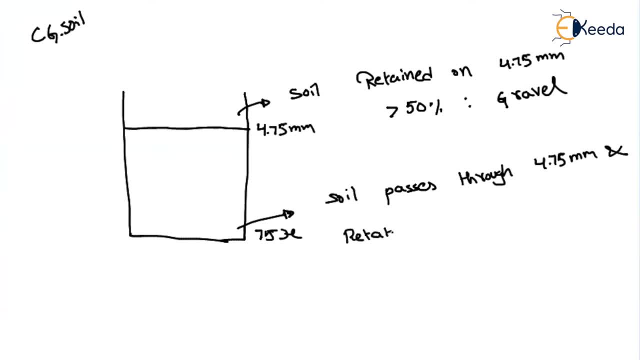 and retained, retained, on which one retained on 75 micron is greater than 50 percent, then we will classify it as a sand. that means whatever the soil if you are keeping on the sieve, then whatever the soil that is retained on the 4.75. if this percent is greater than 50 percent, we will classify it as a gravel. and 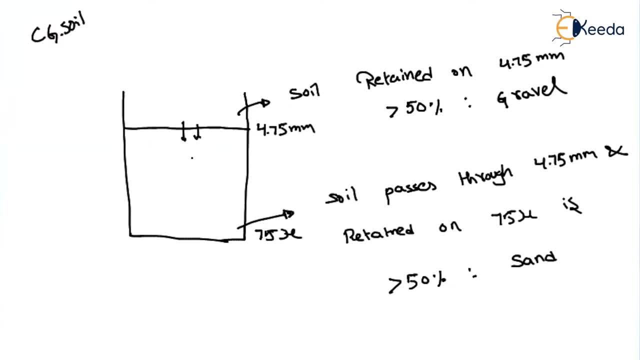 whatever the soil that passes through 4.75 mm and if it is retained on 75 micron- if it is greater than 50, we will classify it as a sand. sir, why can't we simply write it on soil retained on 75 micron? we can't you know why? because if i'm saying the soil is retained on 75 micron, 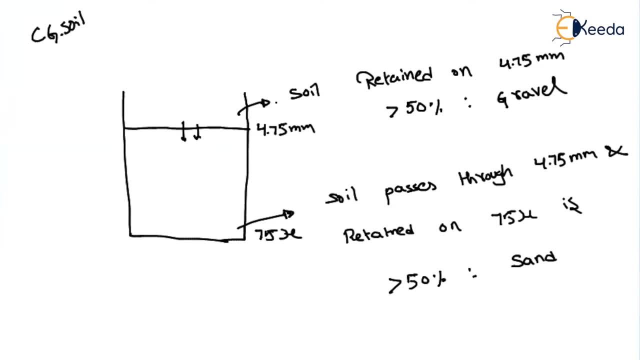 if i don't give 4.75 mm, imagine that means everything will be retained on the 75 micron. so that won't come exactly. so if you want to identify sand, you have to imagine that the soil should pass through the 4.75 and it should retain on the 75 micron. so in the last 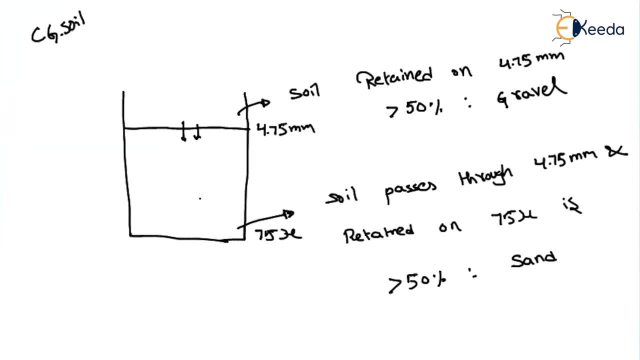 between those two things. whatever the soil is retained, that we will classify it as a sand if it is greater than 150 percent. so let us see with respect to the numericals. so let us say that i have taken thousand grams of the soil. out of this thousand grams, i can say that 800 grams. let us imagine that 800 grams retained on. 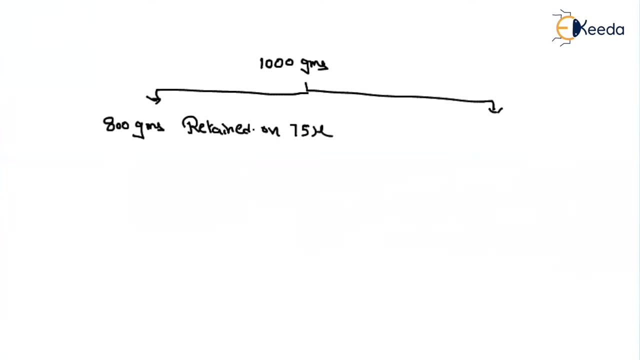 75 micron. so here i am not keeping any sieves, i am keeping only 75 micron sieve. so then, similarly, if it is written on 200, 200 grams passes through 75 micron. so what is the percentage here? and remember that i am using only 75 micron sieve. 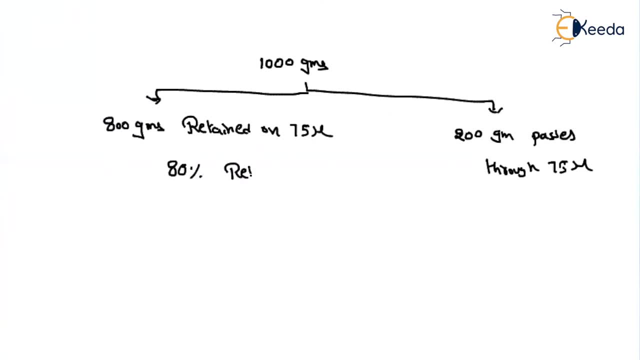 here, whatever the soil is written, 80 percent of the soil is retained and here how much percentage passes. 20 percent is passed, so which is having more percentage? the soil retained on the 75 micron is more so that's why here i am classifying: it is a coarse grained soil right now again, if i 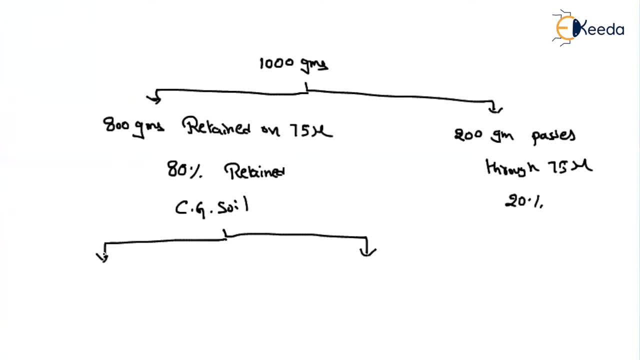 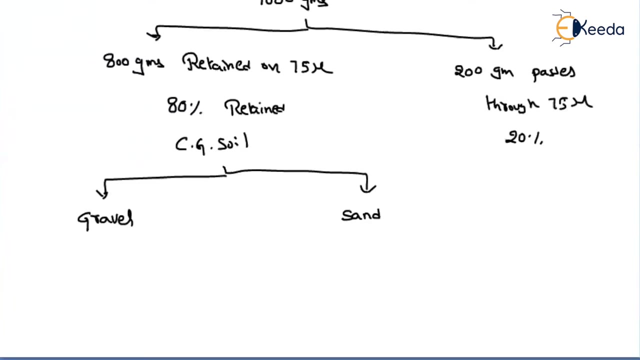 have identified that it is a coarse grain soil and after that, again i have to identify whether it is a gravel or sun. how can i identify it? if it is a gravel, what is the? how can i identify it? if it is a sand, how can i identify it? if it is a gravel? then consider that, imagine. i am just drawing the. 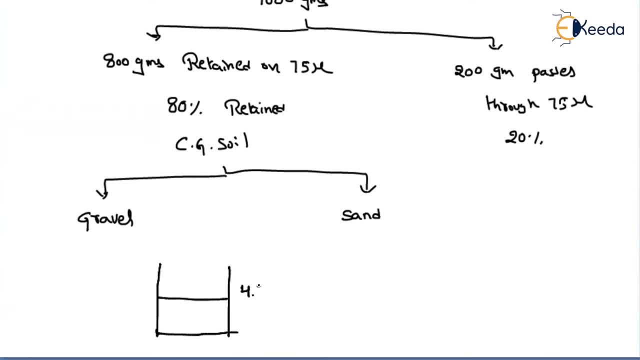 sieve positions. imagine that this is a 4.75 mm and this is the 75 micron. imagine that out of the 800 grams, 300 grams is written on the 4.75 and 800 500 grams written on the 75. so now we are talking about only coarse grain fraction. what is the total coarse grain fraction? 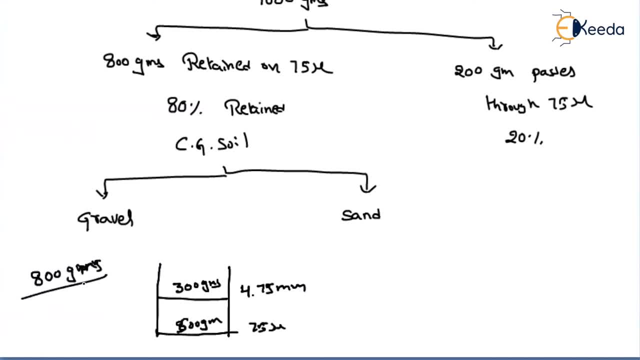 800 mm for 800 grams. so out of this 800 grams, 300 is written on the 4.75 and 500 is written on the 75 micron. then how can i classify it? out of this 800, 300 is written on the 4.75, 500 is written on the 75, so obviously we can say that. 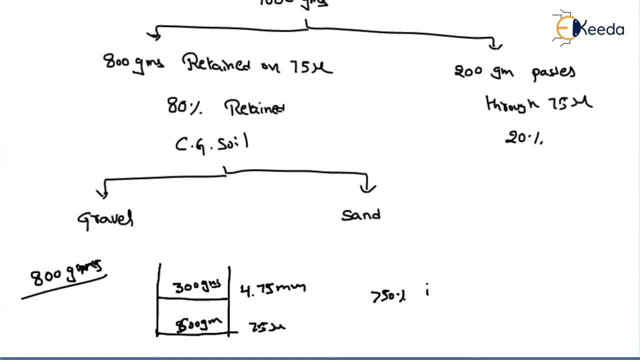 greater than 50 is written on which one greater than 50 is retained on 75 micron. so to consider, greater than 50 percent is passes through, passes through 4.75 mm and retained on 75 micron, then what we can classify? we can classify it as a sand, okay. so first we have to identify that it is a coarse grain fraction. 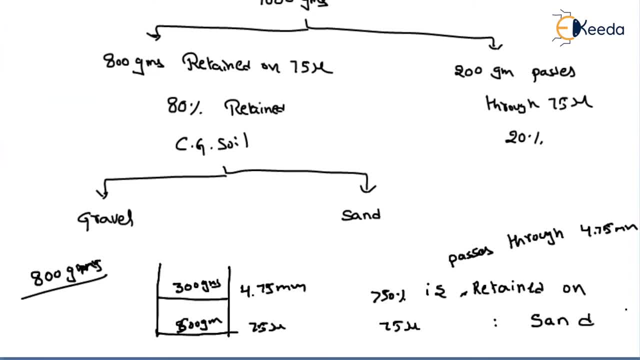 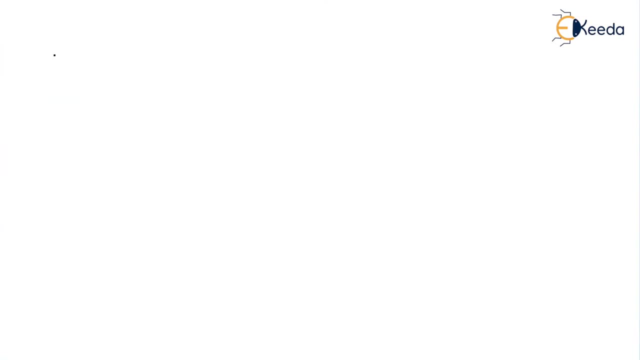 or fine grain fraction. after identifying it, then you should further classify that it will comes under course gravel or whether it comes under sand. okay, now let us say observe that we have identified our present as a gravel, so how can i say whether it is a course well graded gravel? 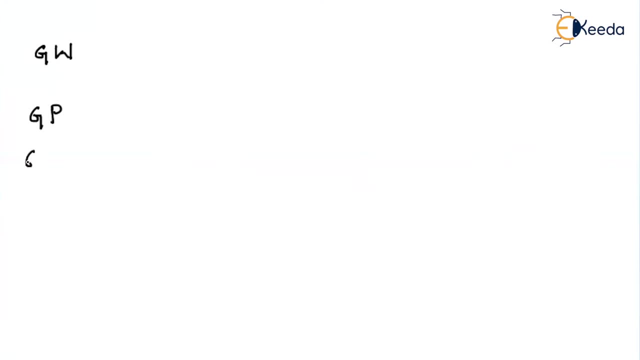 how can i say whether it is a poorly graded gravel? how can i say whether it is a silty gravel and how can i say whether it is a clay gravel? so i will say my well graded gravel, if of my first condition is that percentage of fines. 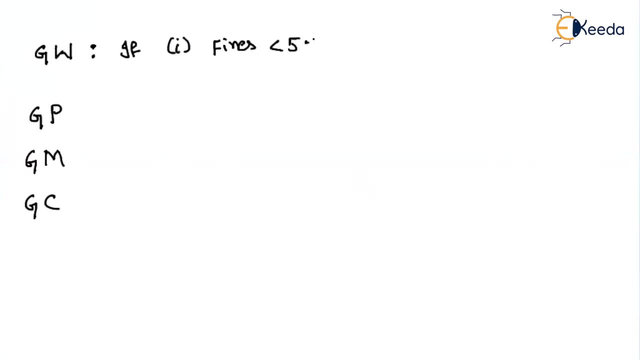 fines should be less than 5 percent. fine is nothing but a soil that passes through the 75 micron mm. micron u. so the soil that passes through 75 micron. if it is less than 5 %, it is a fine level gravel: 5%. and if your coefficient of uniformity greater than 4 and coefficient of curvature value. 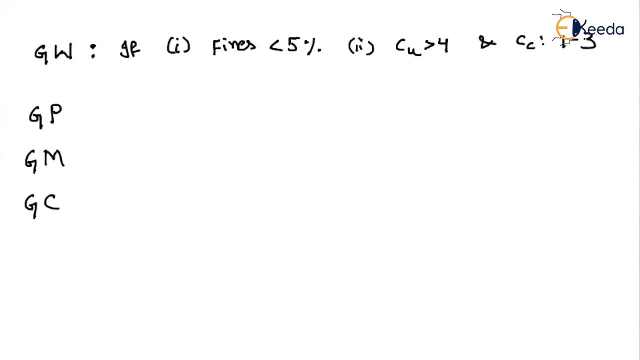 if it is 1,, 2,, 3, then we will classify that as a well graded gravel. Similarly, poorly graded gravel: the first condition is that the fines should be less than 5% and also whatever the second condition if it is a poorly graded, not meeting this requirement. 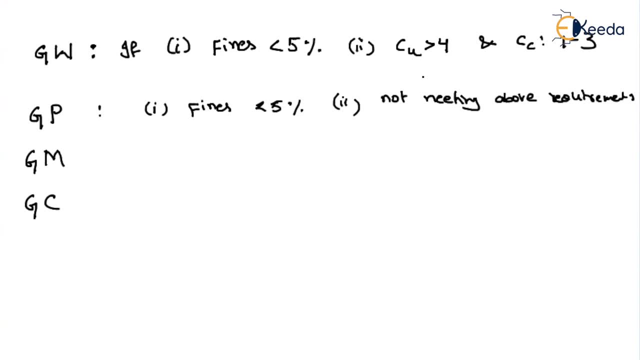 that means if Seiu, if it is not coming greater than 4, or if C C is not be in between 1, 2, 3, if anyone of this not matched, then we will classify it as a poorly graded gravel. 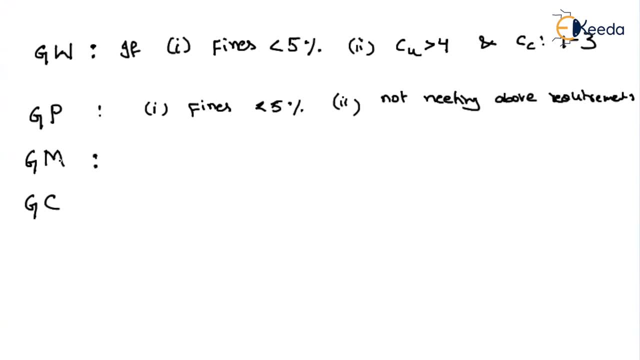 Similarly, we will classify it as a semi graded gravel. So to call this as a newly graded gravel, That means we will classify it as a poorly graded gravel. Similarly, we will classify it as a. similarly, we will classify it is silty gravel when your fines are greater than 50 percent. these are greater than 12 and second. 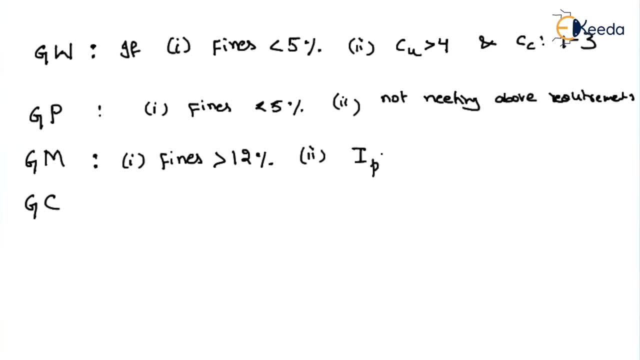 condition is that your ip. ip is nothing but a plasticity index. either you can say if it is less than 4, or you can say it is false, below a line. false below a line. what is mean by alien? i will tell you in minute. so when you will say it is a silty, silty gravel, your 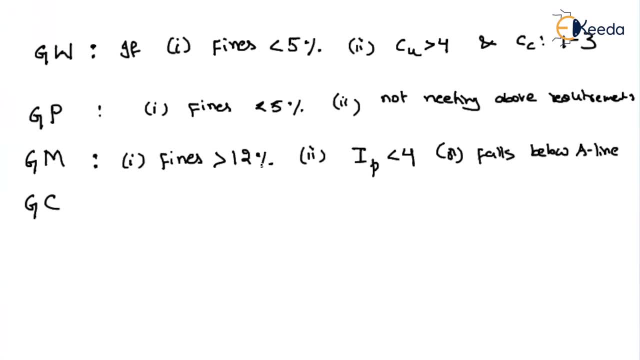 soil passes through 75 micron. that should be greater than 12 and your plasticity index should come less than 4, or it falls below the a line. you can see which falls point. falls below the a line, then we will classify it as a silty gravel. similarly clayey gravel. 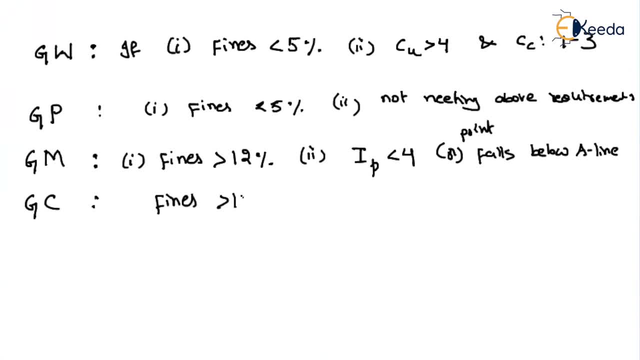 i can say when my fines is greater than 50 percent, so when you will say it is a silty gravel, it is greater than 12. and also i can say that if my ip value, if it is greater than 7 or point falls above a line, a point falls above a line, then we will say that as a clayey. 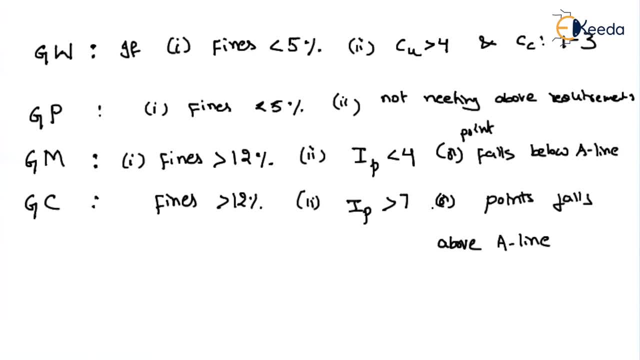 gravel, all these things we have to buy. how did so? if your fine percentage, if you have to check whether it comes below a line or falls below a line or not, well, we can say less than five percent, then we can say that either it comes well graded gravel or poorly graded gravel. 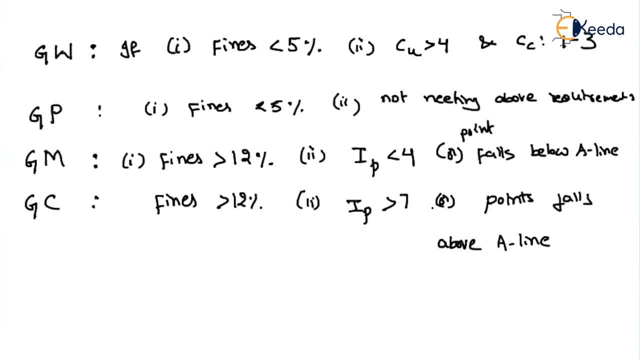 suppose, if your fines are greater than 12 percent, then it will be like whether it may be a silty gravel or clayey gravel. so after identifying whether it is a silty or clayey, then you have to see your ip value and you have to see your a-line diagram. so if it is, point falls below. 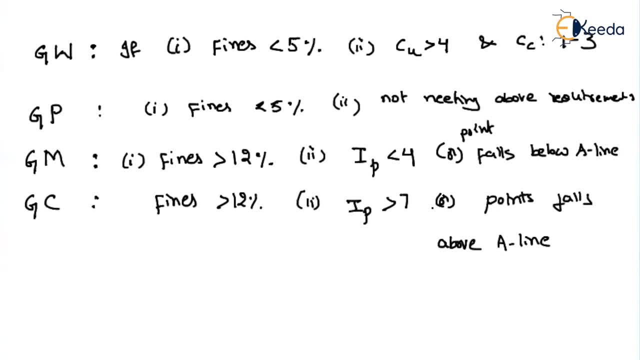 a-line will classify it as a shield. if it is false above a-line, then we will classify it as a clay. so here we have token. let us forgot about this. above a-line, below a-line: here the ip value is less than four. here the ip value is greater than seven. so what about if your ip value comes in? 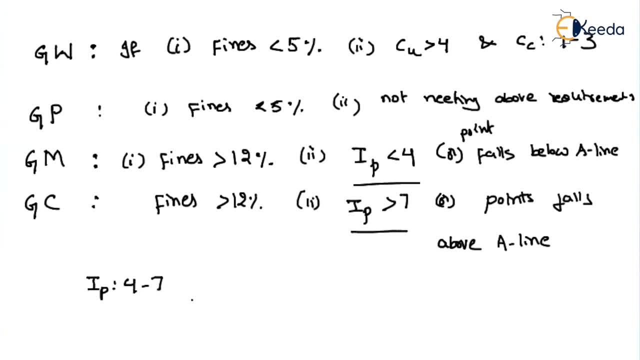 between four to seven if your ip. if it comes four to seven, then we have to say it is a dual symbol. we have to use a dual symbol. that means we will say it is a silty gravel and also we will say it is a clay gravel. so the symbol, 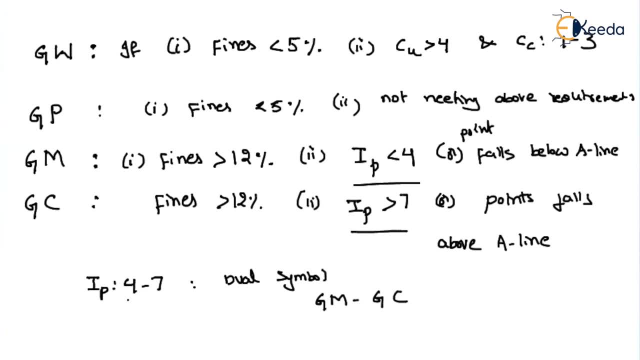 will be g, m to gc. so for four, if it is a less than for, what will classify it is a silty gravel. if it is greater than seven, what will classify it as a gc. so according to this, four to seven also, we are writing this symbol. okay, this is how we are defining the. 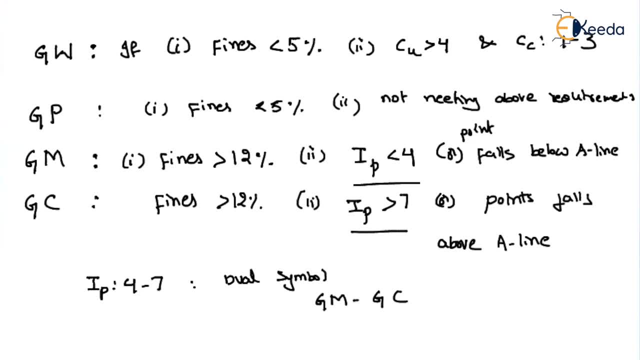 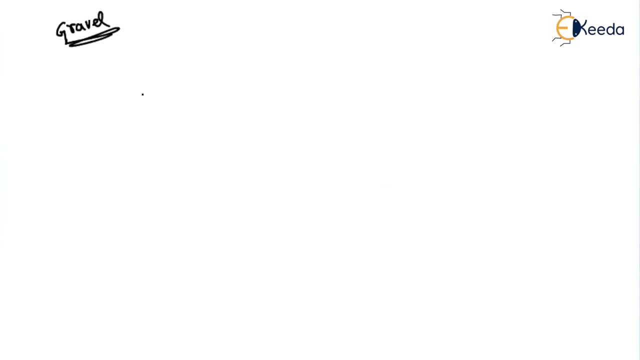 it is a uh for the classification of the gravel. let us take an example. okay, imagine that i am having a gravel soil. let us imagine that i have identified and it is observed that percentage of soil passes through 75 microns is 11 percent and your cu. 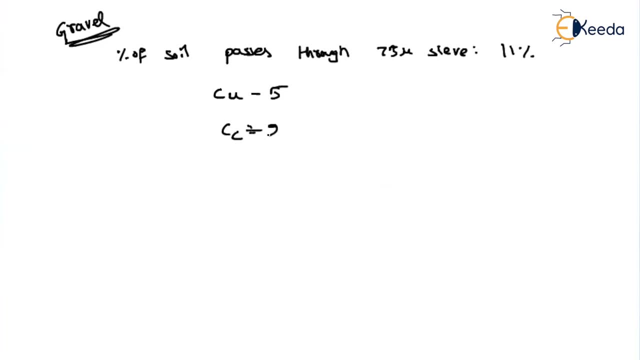 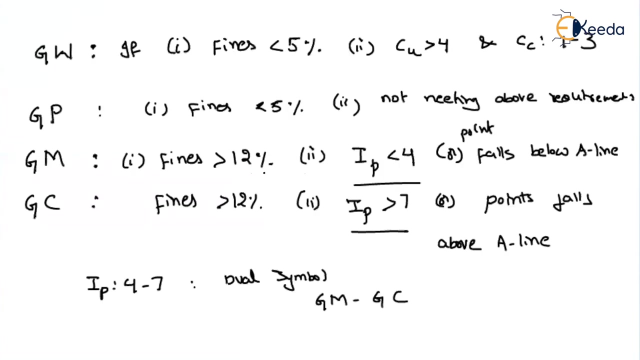 is coming five, and, and your cu is coming five, and and your cc is coming 5, 2 and your IP value is coming 3.. So it comes under which type of the soil? So, percentage of fines: what is the limit? The limit will be 5% and the 12% isn't it. Now we are having 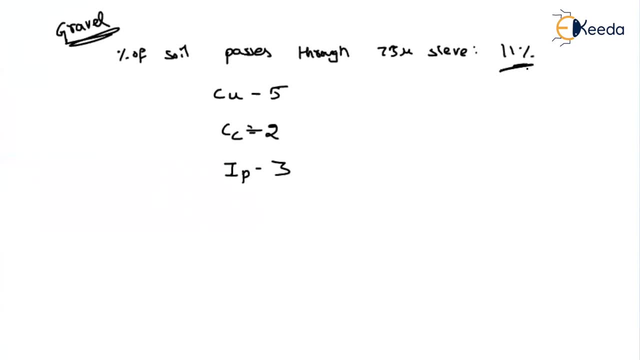 which percentages? So every time it is not mandatory that your fines will be less than 5%, or even fines will be greater than 12%, right? So there might be a possibility that your fines percentage that can be in between 5 to 12 also, Then how can I classify them? 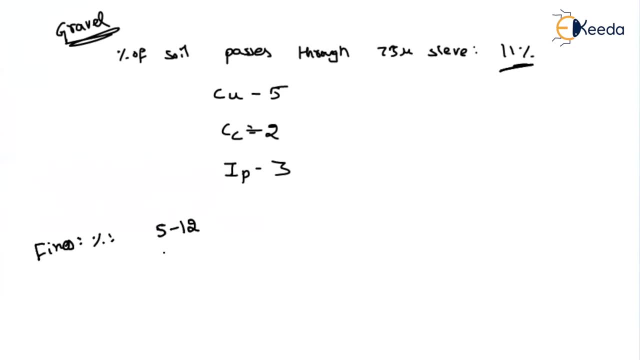 Again, we have to use the dual symbols. Imagine that if it is less than 5.. So how can you classify it? We can classify whether it is a well graded gravel or poorly graded gravel. So how can I identify that My Cu is greater than 4 and my Cc should be 1,, 2,, 3.. My Cu: 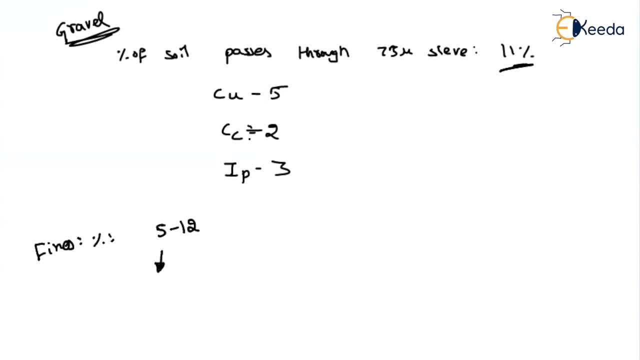 is greater than 4 or not? Yes, greater than 4, satisfied. What about my Cc? It is greater than Cc. It is in between 1, 2, 3.. Yeah, this is also satisfied. This is also satisfied. 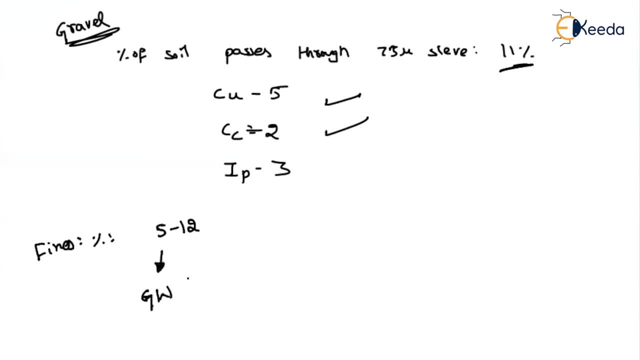 Then how can I classify it? I can classify it as a well graded gravel. So if it is greater than 12, how can I classify it? What about my IP value? My IP value if it is coming less than 3, sorry, if it is coming less than 4 or greater than 7? Less than 4.. That's why. 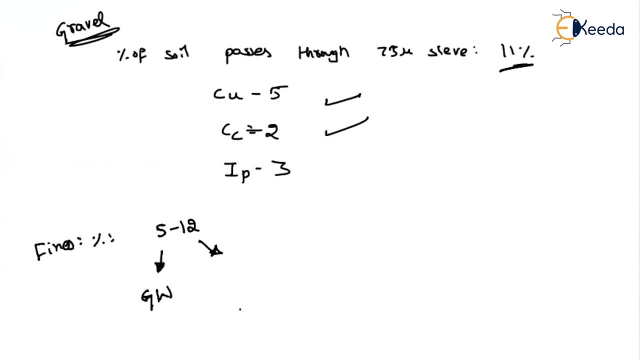 here it will be classified it as a clayey silty gravel. So that's why I should represent GEM. So in the present portion, as my percentage fraction is in between 5 to 12 percent, then I have to use the dual symbol. So if your fines is in between 5 to 12, if it is less, 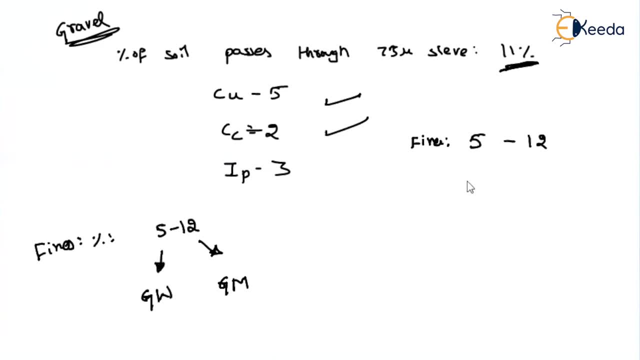 than 5, consider the conditions Which one is satisfying. So, according to the conditions I have obtained, it is a well graded gravel. According to this greater than 12, I have obtained, it is a clayey silty gravel. So as my fines is in between 5 and 12,, I have to use the dual symbol. So if your fines is in between 5 to 12,, then I have to use the dual symbol. So if your fines is in between, 5 and 12, I have to use the dual symbol. So if real value is in between 5 and 12, then I have to. it is a well graded gravel, etc. So what about my present soil? It is. 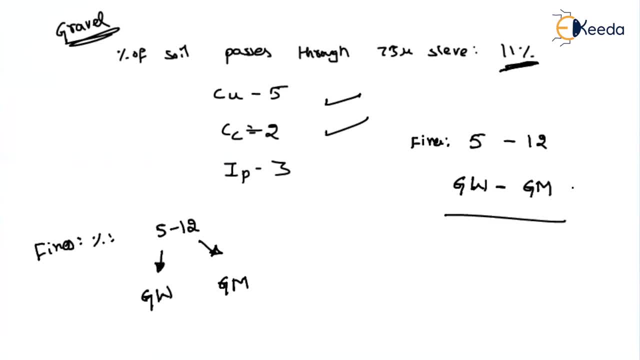 a dual symbol: Well graded gravel to silty gravel. So this is how we have to find out wherever your value is coming in between the portion. Okay, this is how we will classify the gravel soil. Similarly, can you guys tell me how can I classify this sand? Again, the 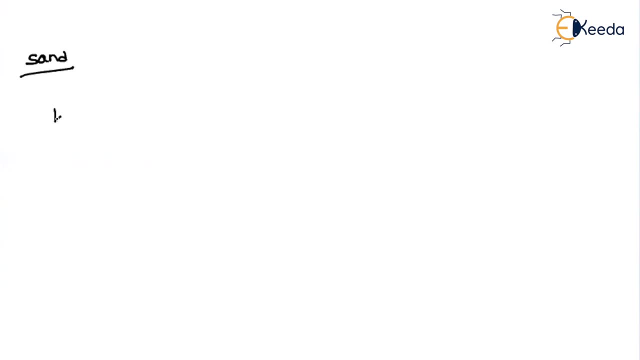 sand. how can I classify why we are classifying Well graded sand, well graded sand, poorly, poorly graded sand and silty sand, and also they're classifying it as a clayey sand. so again, how can i say it is a well graded sand? for that your fines should be again the same. 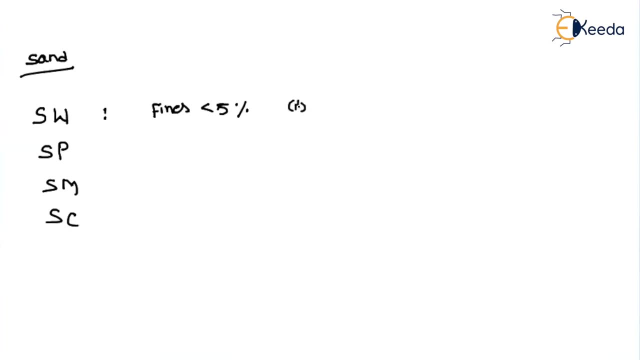 condition, less than five percent. and the second condition is cu. in the previous case, if it is a gravel- well graded gravel- your cu should be greater than four. if it is a sand, it should be greater than six. and the second third condition, cc should be in between one, two, three. 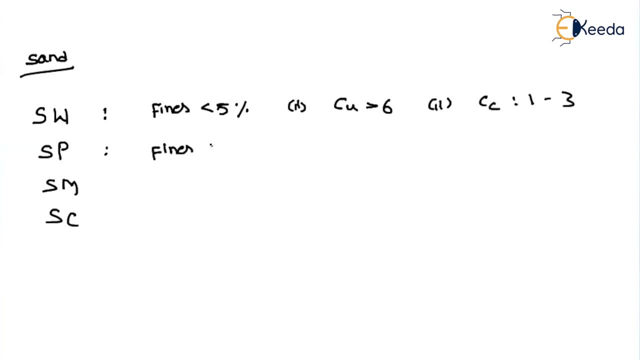 similarly for the poorly sand, your fines should be less than five percent and not meeting above values. that means you either if your cu is not greater than six or your cc may not be between one, two, three, not meeting above requirement. and how can i classify it is a silty sand. again the same condition. 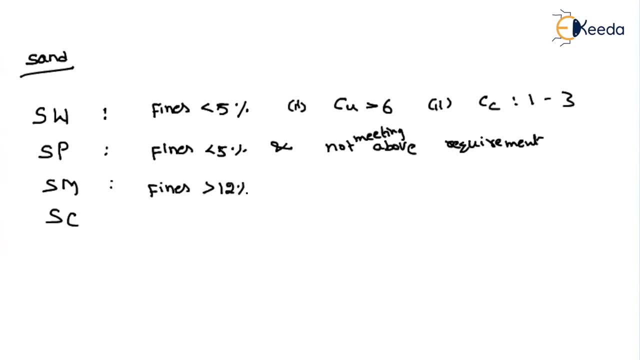 your fines should be greater than twelve percent and your ip value should be less than four or whatever. the point should fall below a line. similarly, what about clayey sand? again, your fines should be greater than 12 percent and your ip value should be greater than seven. 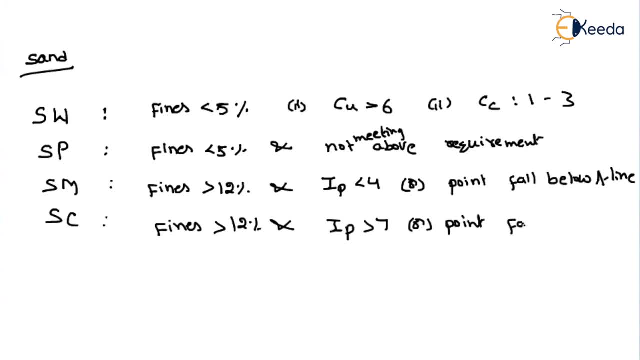 or the point should fall above a line. so this is how we will classify that same. so the conditions are same. only the thing is that here cu values changes, so, but rather than that, all the values will be remain same. okay, in the next video we will discuss about the classification of the fine grain soil. thank you, you.